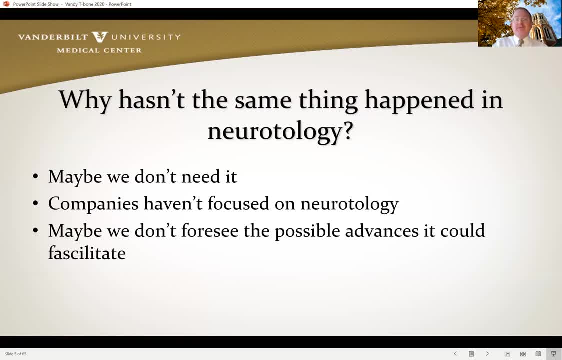 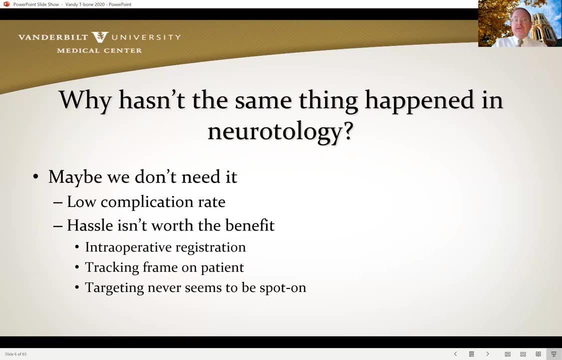 but here are a couple possible reasons. Number one: maybe we don't think we need it. Number two: companies haven't focused on neurotology. Number three: maybe we don't foresee the possible advantages that it could facilitate. Why don't we think we need it? We have low. 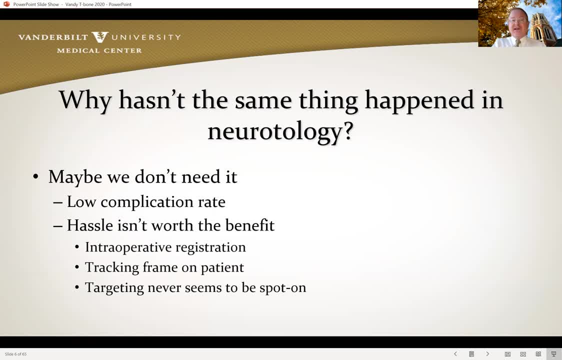 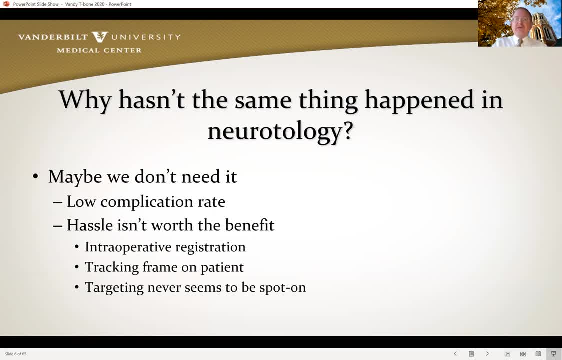 interoperative registration. I've got to set up the interoperative registration. I've got to put this tracking fame on the patient Targeting never seems to be spot on. Interestingly enough, these are the same things that came up in rhinology many years ago. Certainly, companies have not. 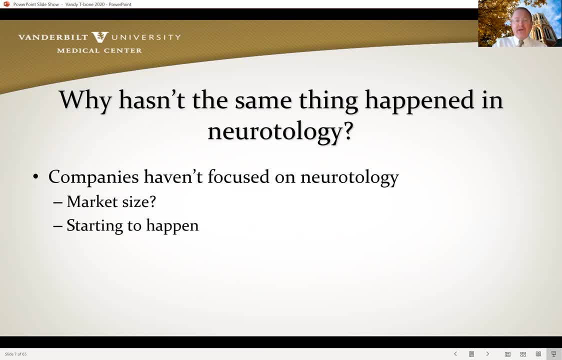 focused on neurotology. I'm not sure why that hasn't occurred. I think part of it is market size, but I do see it starting to happen. And finally, maybe we don't foresee the possible advances it could bring. I'm going to talk about two such advances: customized surgical approaches. 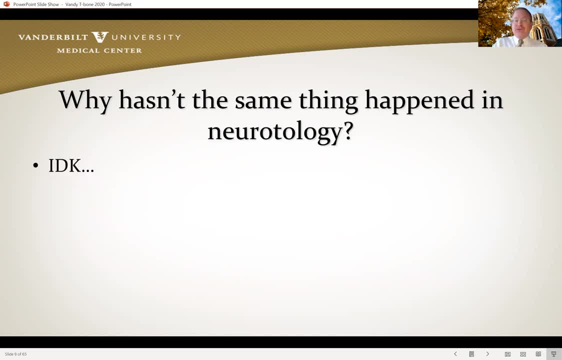 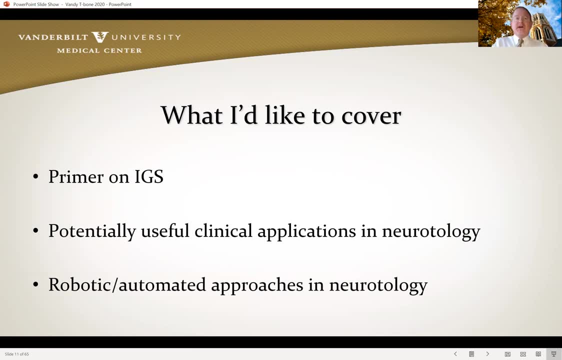 and robotics. So still don't know, but I think it's inevitable that it will happen and we have to be prepared for that. Here's what I'd like to cover today. While we don't have enough time to do an in-depth dive into image-guided surgery, I'd like to do a primer on that and cover certain. 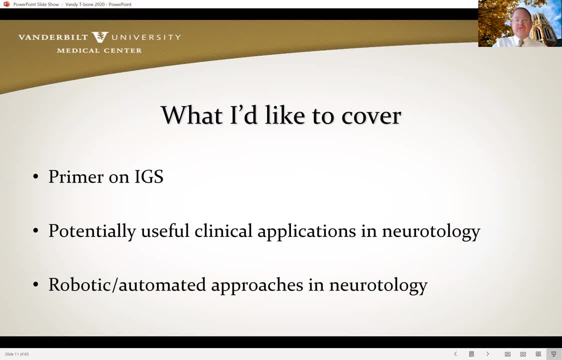 basics that are really important to understanding the accuracy of these systems. Next, I'd like to share two clinical applications in neurotology and bring up others that I think other groups are working on, And then I'd like to talk about the clinical applications in neuroendocrinology. 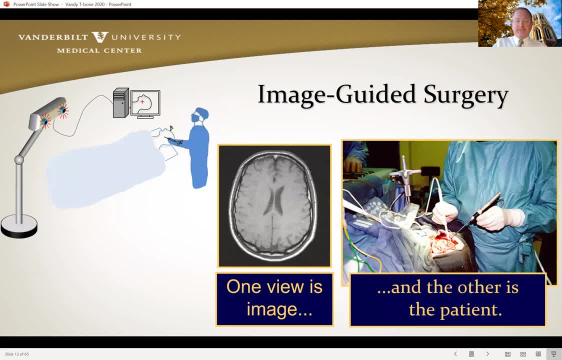 I'd like to talk about robotic slash, automated approaches, Image-guided surgery. I think we all get it. It's kind of like a GPS in the operating room. You have a TRAX instrument where the surgeon touches a spot on the anatomy and it shows up, typically on an MRI or a CT scan and a monitor. 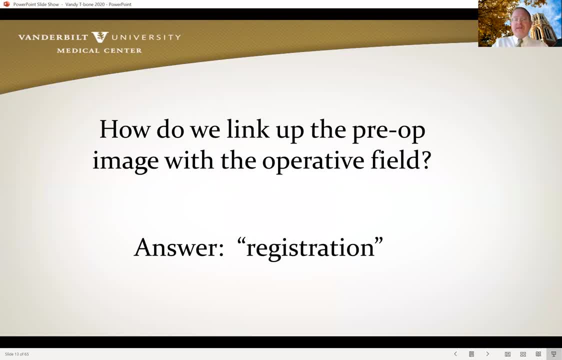 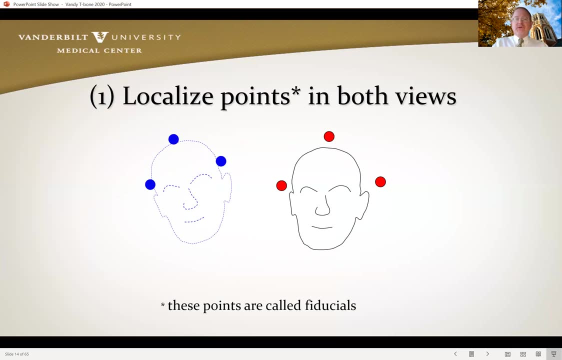 in front of the surgeon's view. How do we link up the anatomical anatomy to the MRI or CT scan? The answer for this is registration. Registration is the key piece of image-guided surgery. What we need to do is identify points in both the x-ray view shown in blue and in the physical space in the operating room shown in red. 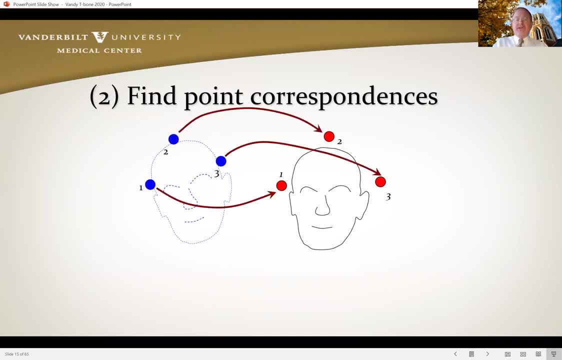 These points are called fiducials. You find point correspondences one, two and three in x-ray, one, two and three in the operating room, and then you have to align these up. How do we align them? First you have to rotate. 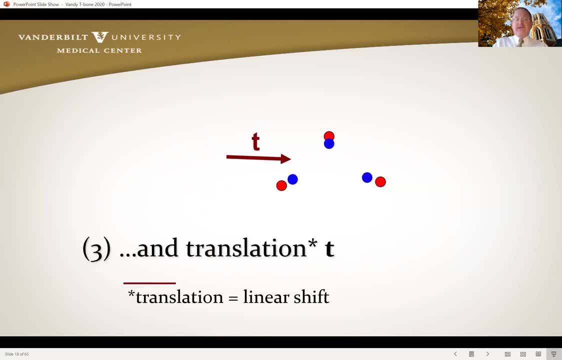 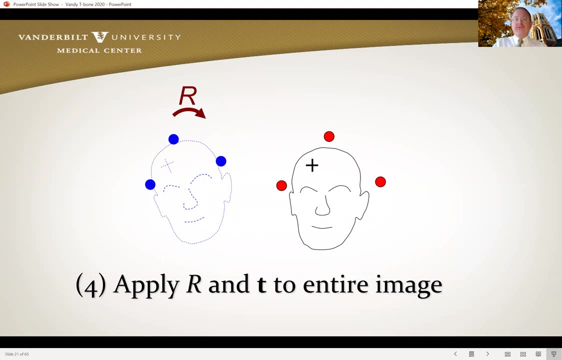 The whole space And then you translate that space in a manner that will best align the fiducials. And for my engineering colleagues out there that best alignment is a least squared alignment error. Once you do that with those fiducial points, you do it to the entire images. So all of the dependent 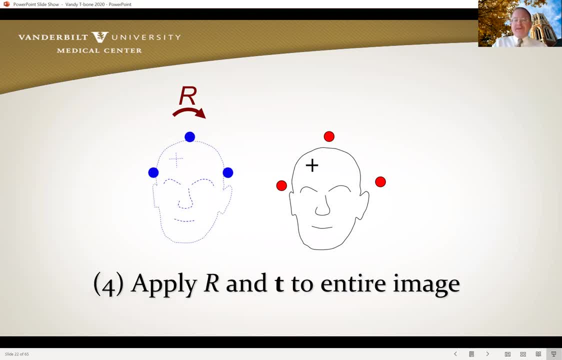 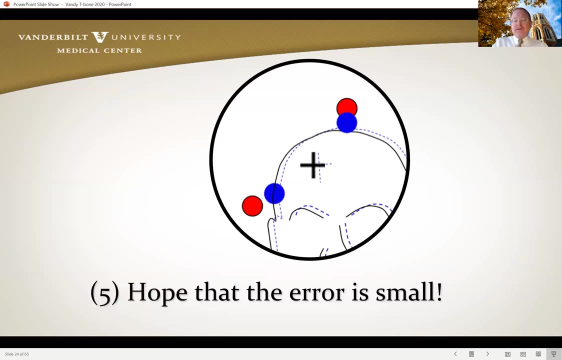 anatomy comes along for the ride And once this occurs, you quite frankly hope that the error is small and that it will be clinically useful to you. So if you look at this mark on the forehead, the x is where you want it to be, the dotted lines are where it says you are and you hope that that. 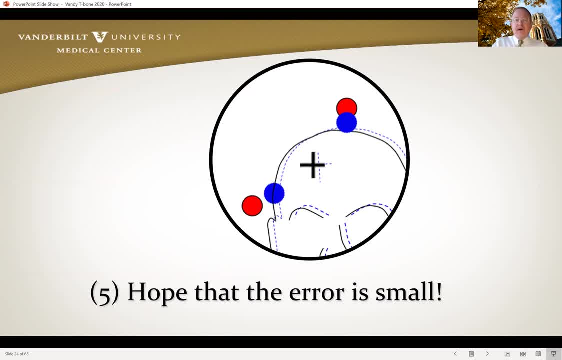 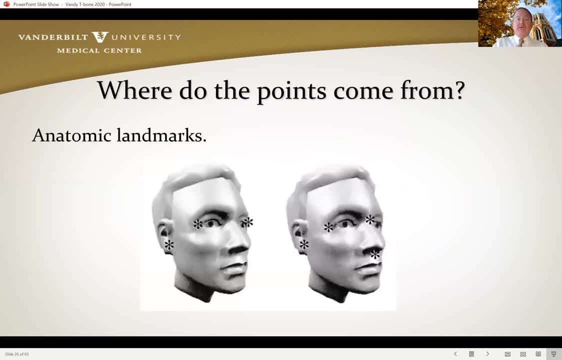 error is very small and that it will be helpful in you making clinical decisions in the operating room. So how do we localize points on the patient? We can use anatomical points. The problem with this is that they're very hard to reproducibly find. You can't always be in the same spot each time. 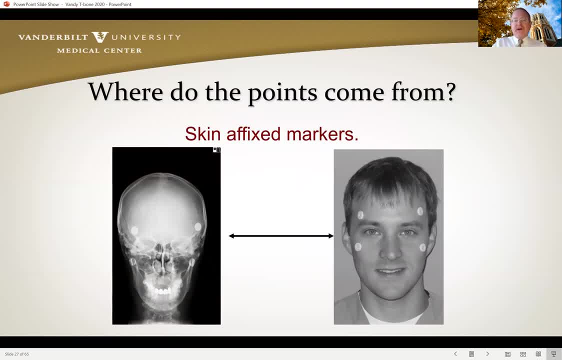 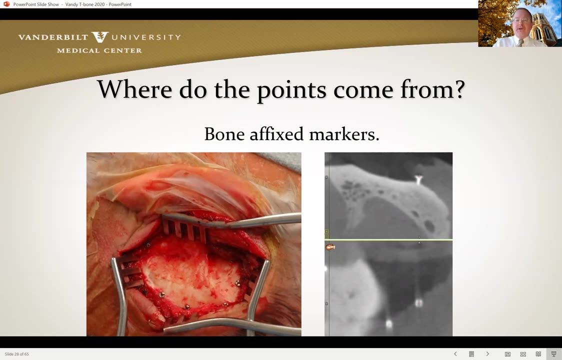 We can use skin affixed markers. You can always find the skin affixed marker but the skin moves relative to the skull So that introduces error associated with it. Really, for neurotology and neurosurgery the best things are bone affixed markers And they can be as simple as these facial 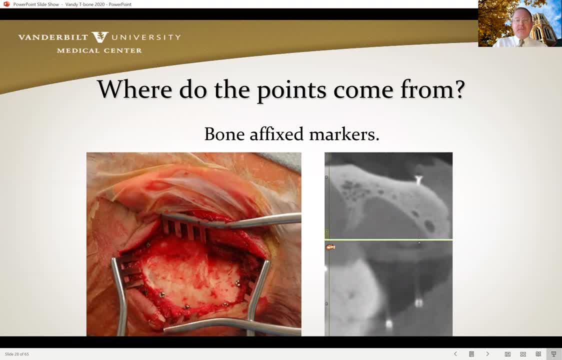 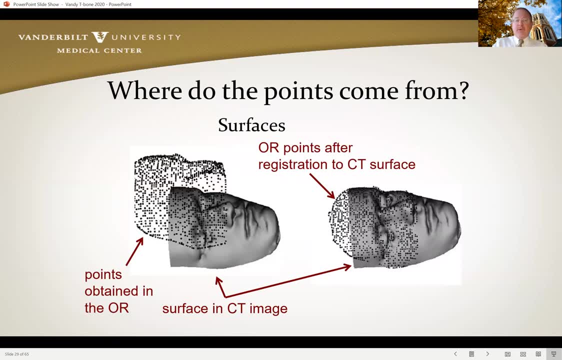 plating screws placed in the lateral skull base. The minimum number you need, of course, is three to get three-dimensional localization. The most common way our rhinology colleagues do this is surface mapping. So they'll take a laser probe or they'll take a tract probe and rub it over the 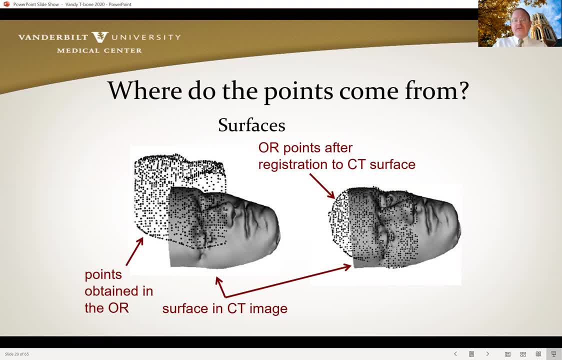 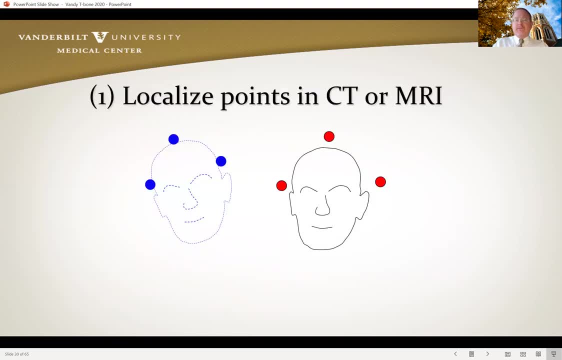 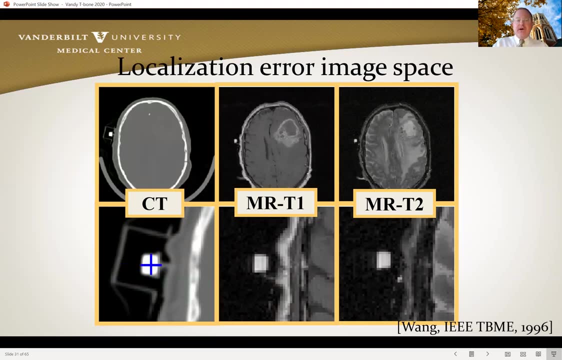 prominences of the forehead and the nose, and then you can find those same contours in the CT space and then align the two. How do we localize the points in CT or MRI? Well, you actually have to do this, You actually have to pick them out, And that's easier said than done, because image space is. 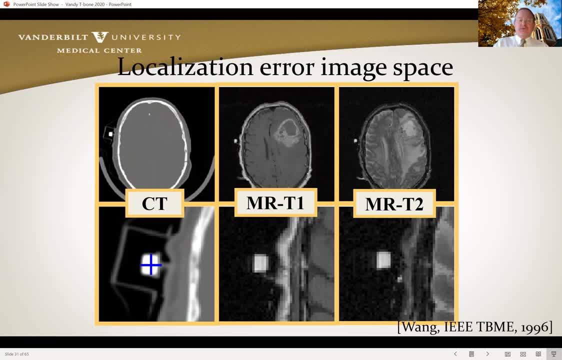 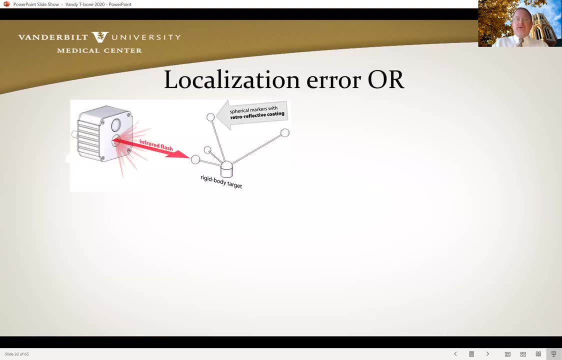 created of pixels or more appropriately, voxels, which are three-dimensional pixels And you can see in the CT and in these MRI spaces. it's not always perfect in taking the crosshair and putting it on the center of the fiducial marker. When you localize in the OR, you're using typically an 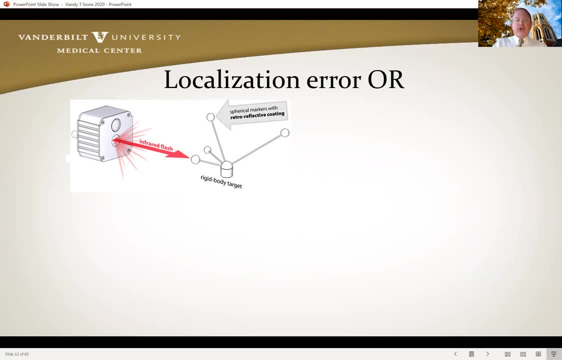 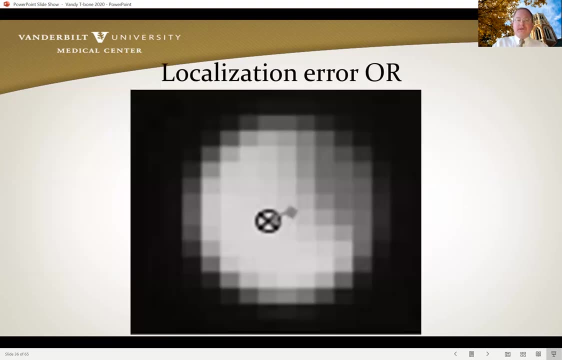 infrared tracer- You can also use EMF, but I'll show it here- for infrared- which shines a light on an ultra-reflective marker That reflects back and is picked up by the camera which can then find the centroid of those markers. Problems with that are if there's a smudge on the marker, If you have blood on your gloved. 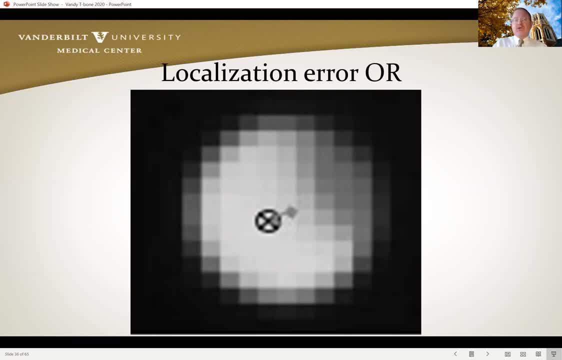 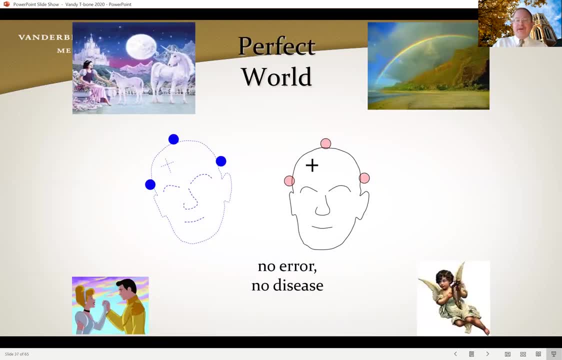 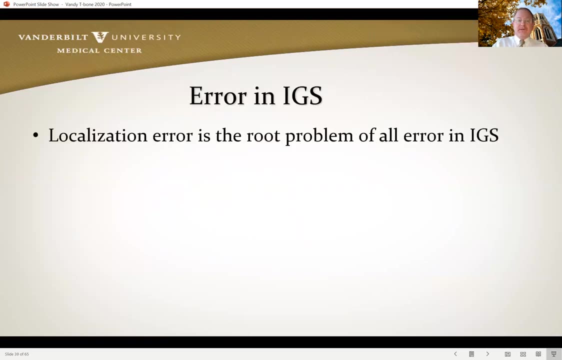 hand and you touch the marker, it can erroneously distort it to the IR camera. So in the perfect case you can find everything up and there is no error. But in the real world things don't work that perfectly. So localization is the root problem of all errors in image-guided surgical. 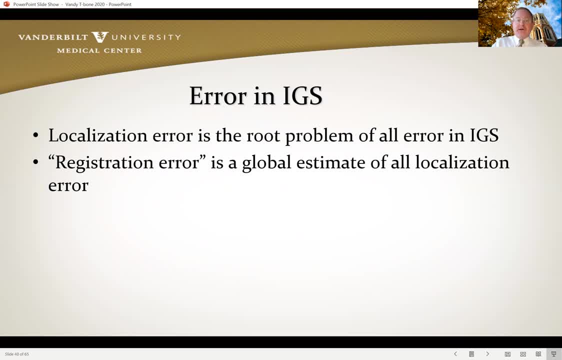 systems. There's another term called registration error, and it's a global estimate of all localization error. It is typically what the machine tells you once you've registered in the operating room, Usually improves with more markers, and it improves with more markers So you can. 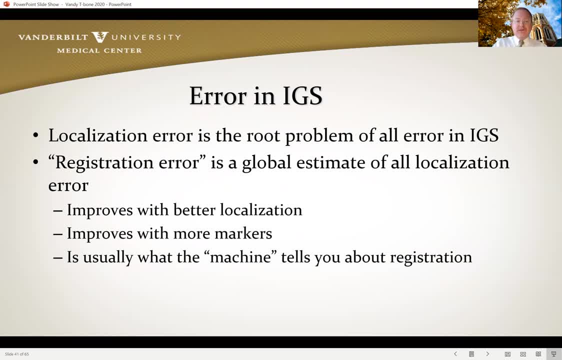 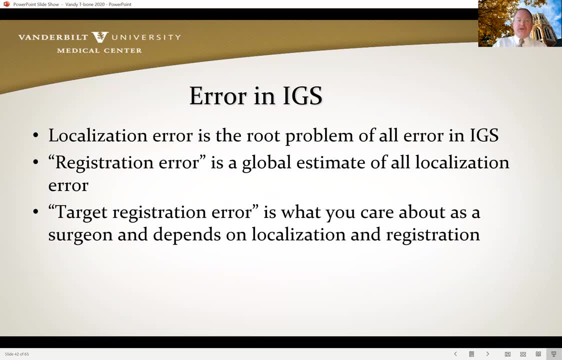 use with better localization. So it all comes down to the localization of the markers. Target registration is what you really care about as a surgeon. It's the accuracy of the system. It is the difference from putting the marked, the tracked probe, on a spot and what that spot should. 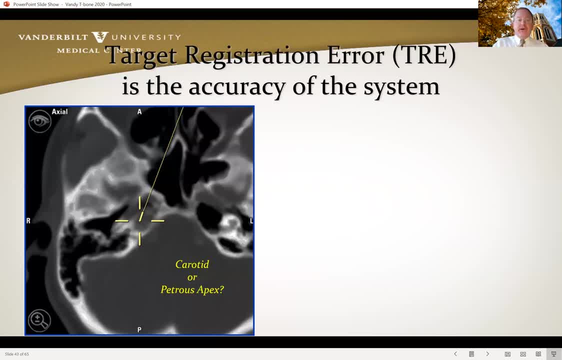 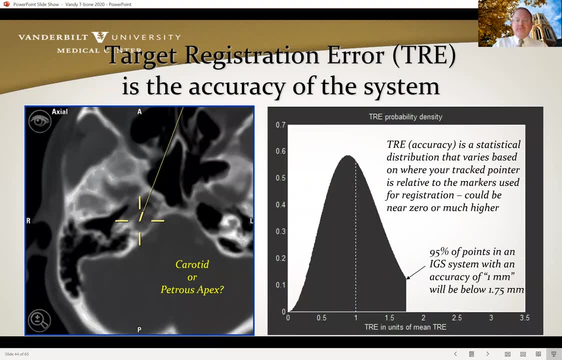 be in the CT or MRI. So, for example, here we're touching what we hope is Petrus apex, but it's telling us we may be in the carotid artery. Now, the deal about accuracy of a system is that there isn't one number, It's a statistical distribution. 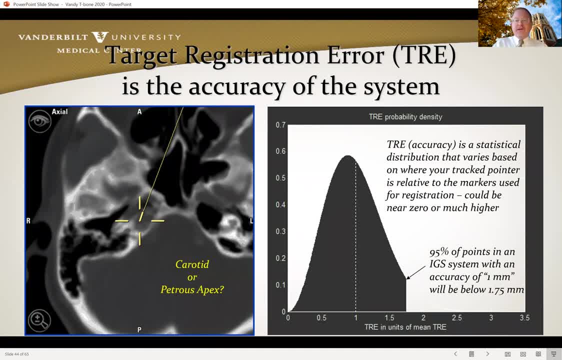 that varies based on where the tracked pointer is relative to the markers used for registration. So it can be very close to zero or it can be much higher. And this statistical probability shown on the right side of the screen. this is a system that claims an accuracy of one millimeter. 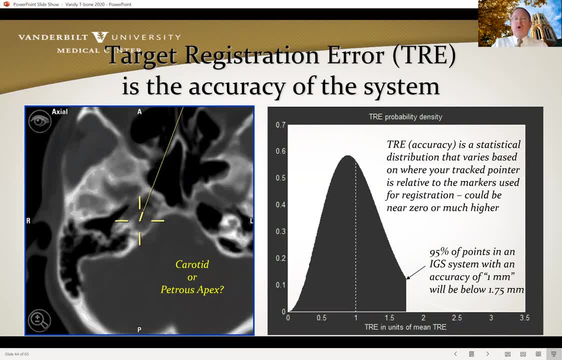 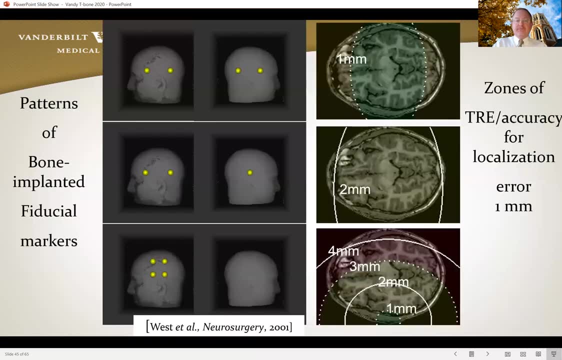 And the accuracy of that accuracy is about 25 percent of those points will be below 1.75 millimeters, but some will be higher. So you can have accuracy in this system as high as 2.5 millimeters, based on where you're tracking at that moment. in reference to the fiducial markers, 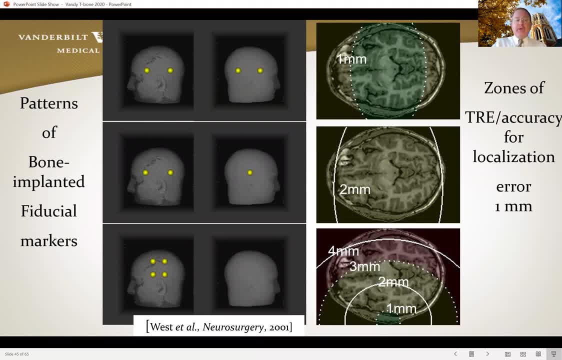 Here's an example from neurosurgery that shows how important where you place the fiducial markers is. On the left-hand side of the screen you can see the gold markers. On the top panel you see two markers on each side of the head. On the right side you can see what the zone of accuracy is. 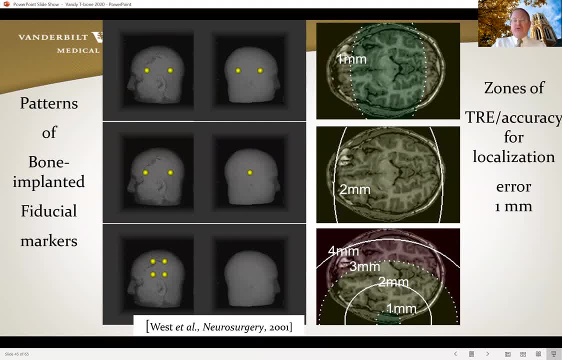 So the zone of accuracy would be less than one millimeter for the vast majority of the intracranial space. for this example, In the middle panel you can see two markers on one side and one on the contralateral side, And this makes the zone of accuracy about two millimeters for that intracranial space. 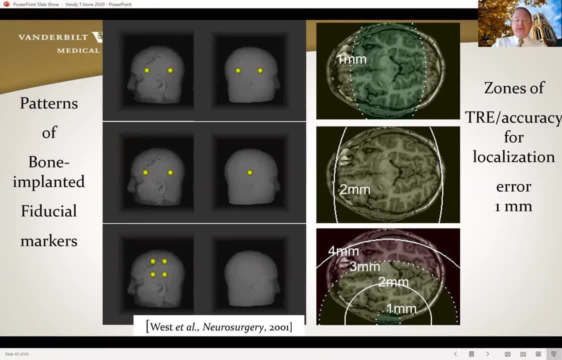 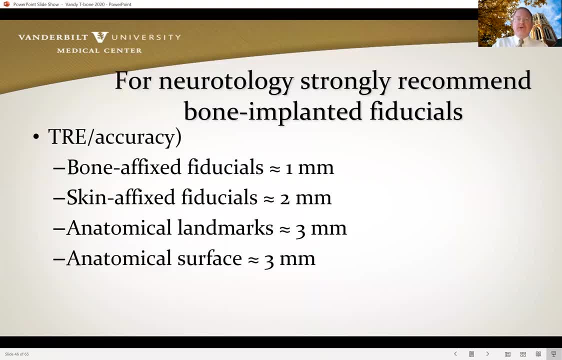 And then if you have four markers on one side, you have very good accuracy near that surface, But as you go deeper into the brain it gets worse. So for neurotology we really need to use bone implanted fiducials. Skin affixed fiducials produce accuracy in a system of about two millimeters and anatomical landmarks about three millimeters. 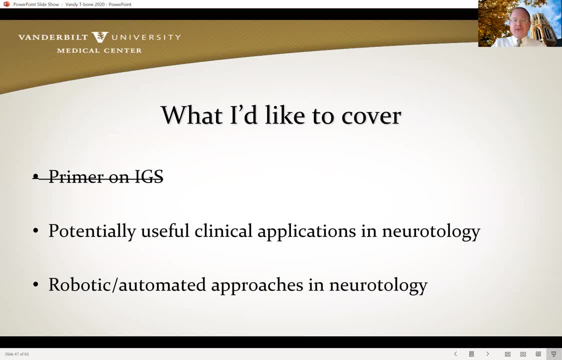 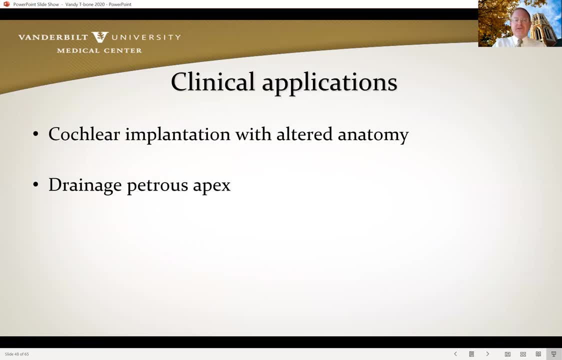 So hopefully that gets the point across that localization and registration of these systems is vital for us as surgeons to understand. So how about some clinically useful applications in neurotology? First, cochlear implantation with altered anatomy and second, drainage of a petrous apex lesion. 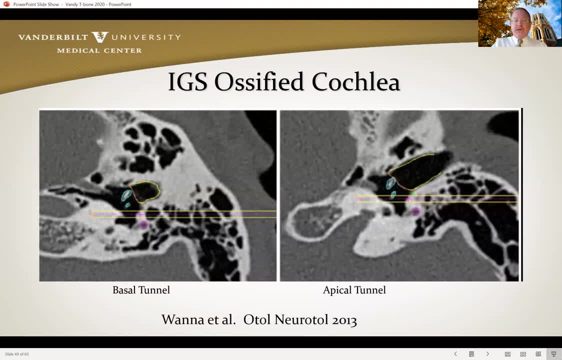 So this is an interesting case of an ossified cochlea. You can see on this temporal bone CT scan that you can't see anything that resembles a cochlea because it has been completely ossified. For these type of situations we typically will do a split electrode array. 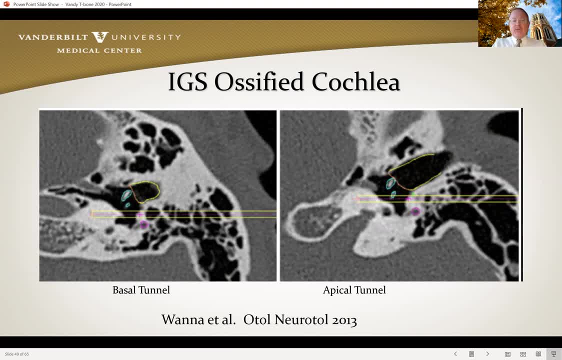 or we'll try to put one electrode array in where the basal turn was located and the other in where the apical turn was located, In the hopes of surrounding the medialis and causing some stimulation to the eighth cranial nerve. This is a case that was done with a formal faculty member, George Juana. 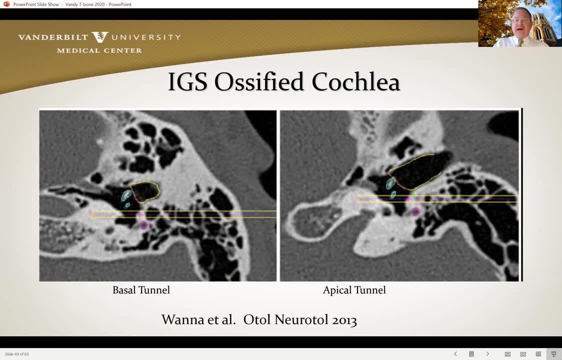 And you can see on the left side the basal tunnel that's planned out preoperatively, And then on the right side, the apical tunnel. We were able to achieve these tunnels only with the use of image guidance. To do this without it would have been a complete shot in the dark. 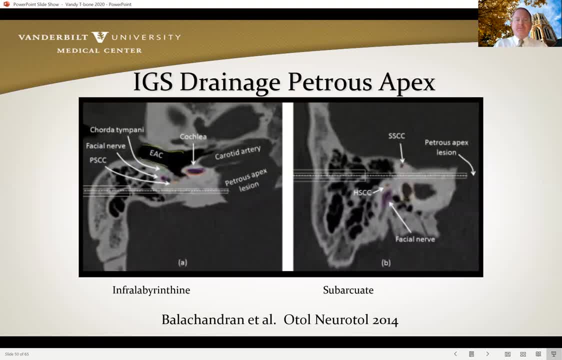 Here's another example- This is an interesting case- which is drainage of a petrous apex lesion. This was done with current faculty member Mark Bennett And you can see that we planned out an infer labyrinthine approach on the left side and then a sub arcuate approach right through the superior semicircular canal on the right side. 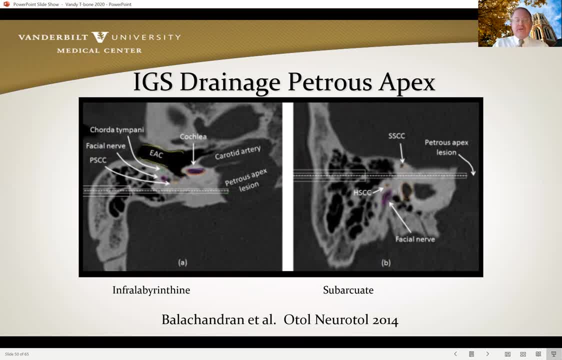 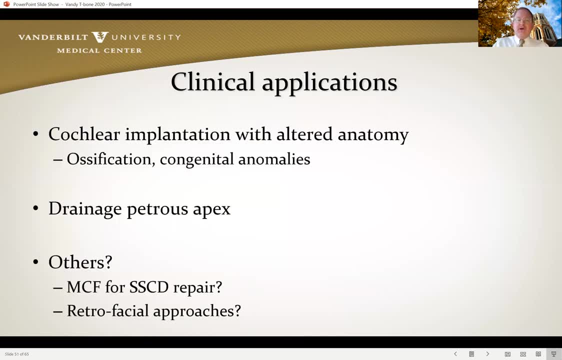 Using image guidance, we were able to achieve these trajectories and able to drain this lesion and actually irrigate through one port and suction through the other. Now I know there are a lot of other image guided surgical applications. some that quickly come to mind are: middle cranial fossa approach for superior semicircular canal dehiscence. 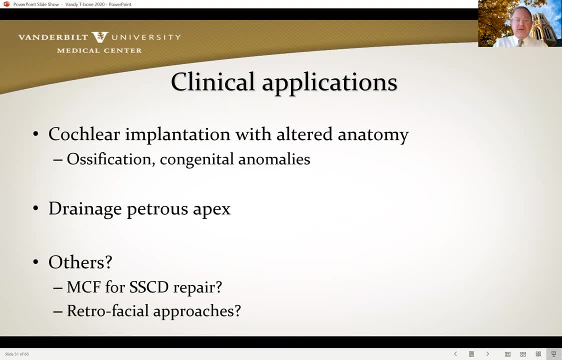 I know that some groups are working on this and actually do this routinely. And then you start thinking about novel approaches. Can we do retrofacial approaches? Can we get to certain areas of the anatomy where we think disease may be hiding, but right now we might not have the confidence to approach them because of the risks of damaging vital structures. 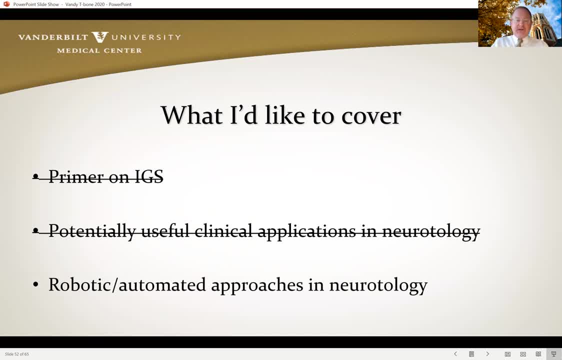 What's in the future? Well, certainly, image guidance is going to allow us to do robotic and or automated approaches, And I'd like to share two with you that we're working on right now. The first is minimally invasive image guided cochlear implantation. 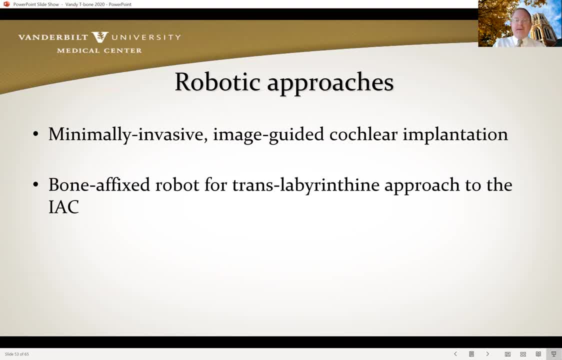 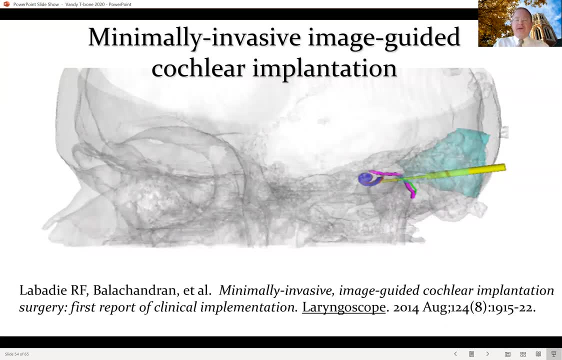 And the second is a bone affixed robot for trans labyrinthine approaches to the internal auditory canal. So the concept of minimally invasive, image guided cochlear implant is that, instead of doing the mastoid, which was really an access surgery, you plan. 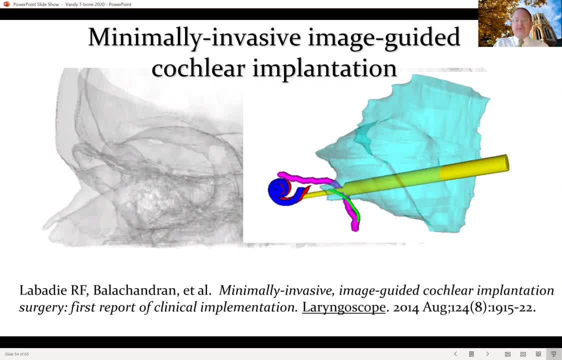 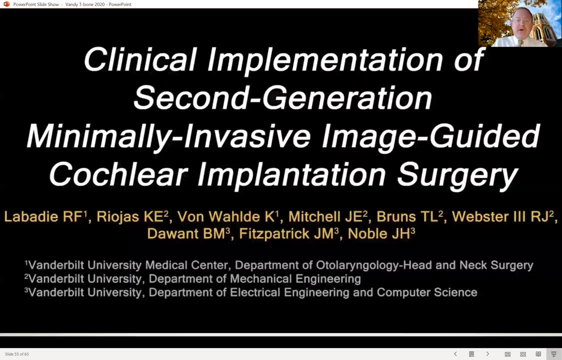 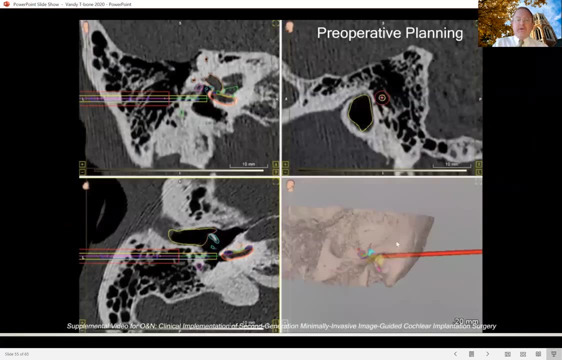 and realize a linear tunnel from the surface of the mastoid through the facial recess to the basal turn of the cochlea. This is a video from a paper that is in press at Otology, Neuro Otology, showing our most current work on this. Here is the planning done on the preoperative CT scan, where we segmented the vital anatomy. 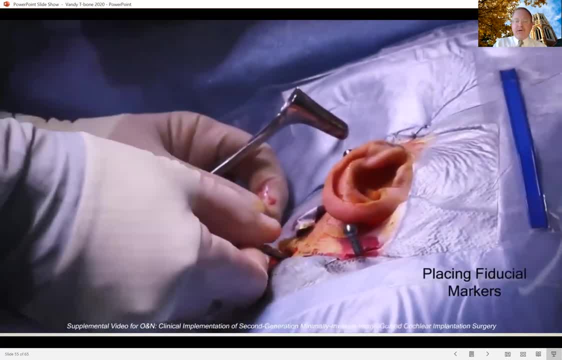 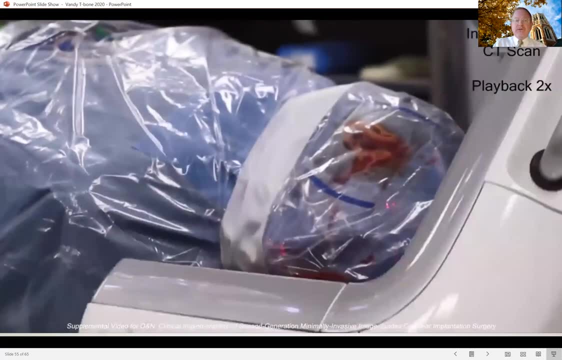 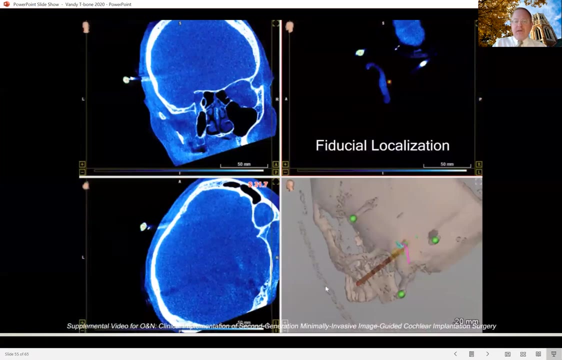 Here I am placing bone implanted fiducial markers- Again bone implanted- so we can get the accuracy that we need. We use an intraoperative CT scan to be able to identify where those fiducial markers are on the CT And then we know where they are in the patient. 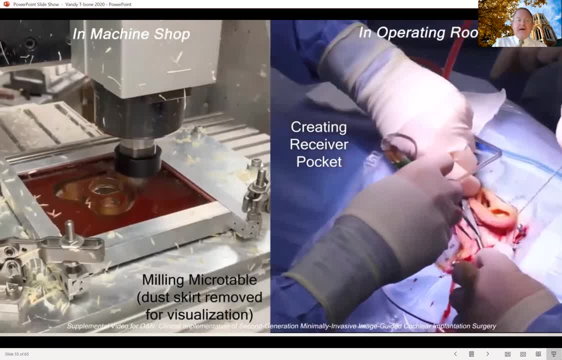 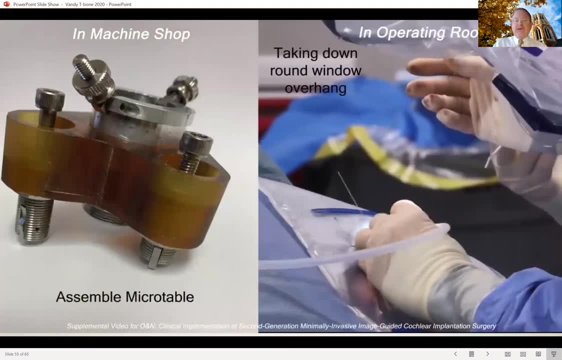 We then make on the fly a customized microstereotactic frame that will mount to those fiducial markers and limit the drill trajectory to the path we've selected. While this is being made, I am doing middle ear work to take down the round window overhang. 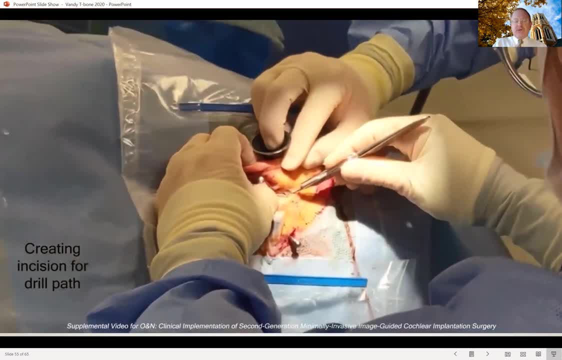 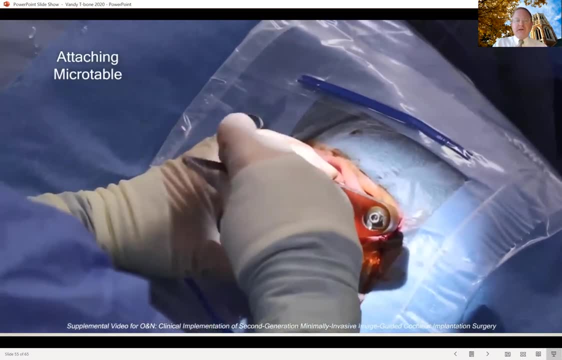 And I am doing some skin incisions so that the drill can contact the bone, and also for the internal receiver of the cochlear implant. Once the microtable has been sterilized, it's passed onto the surgical field and it's secured to the fiducial markers. 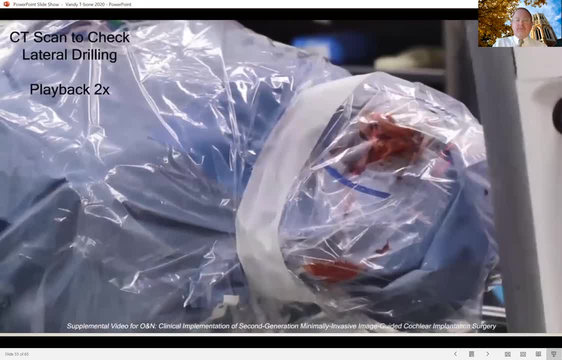 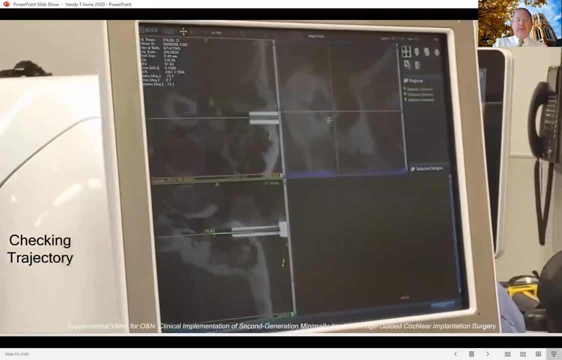 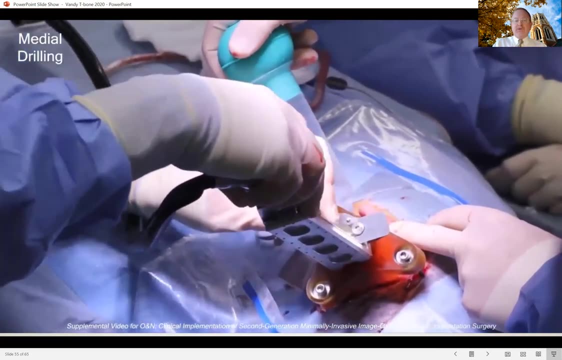 We do a two-stage drilling: laterally with a larger bore drill bit, following which we take a CT scan to confirm that we are accurately targeting the basal turn of the cochlea and avoiding the facial nerve. Then we do a more medial drilling, a pec drilling, where we do incremental tiny pecs with irrigation in between. 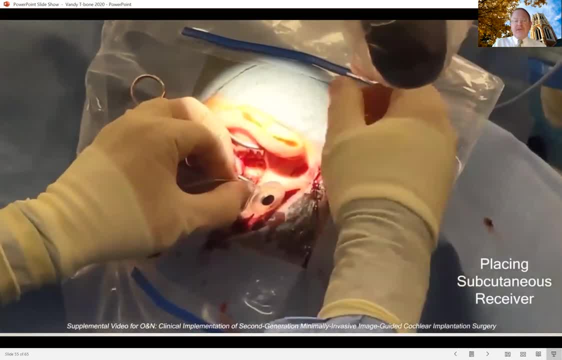 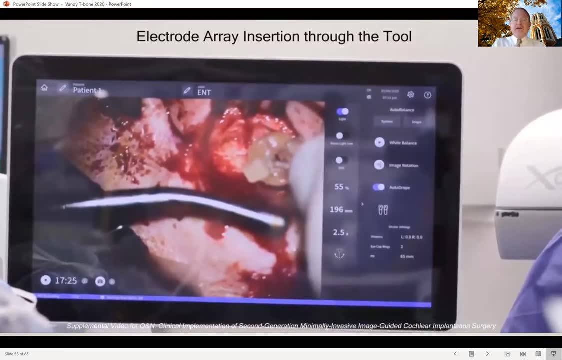 to limit the heat generation. Then we open the cochlear implant from the OR stock, We place it in the subtemporalis pocket, We put the electrode array down the tunnel using a specially designed insertion tool And then we do a final CT scan before we close. 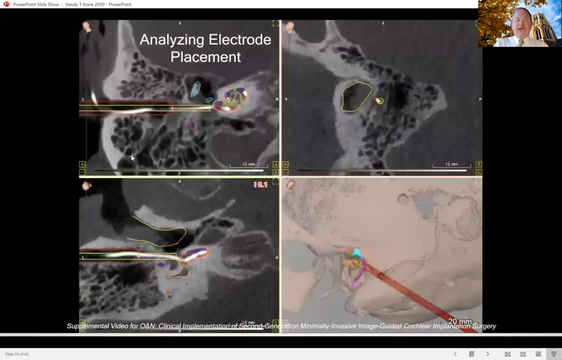 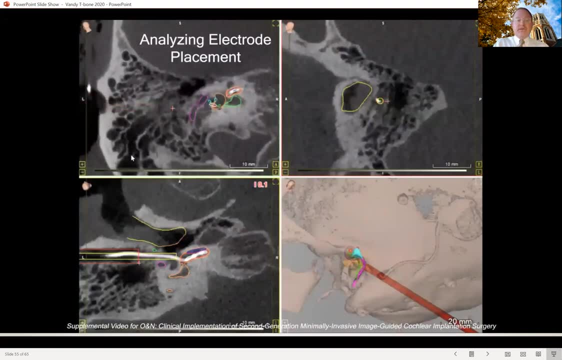 to confirm that the electrode array is indeed in the cochlea And you can see on this image that there is no mastoid drill, There is strictly a tunnel. So that tunnel replaces the mastoid, because we don't need the mastoid anymore, because we're using computer vision with the image guidance. 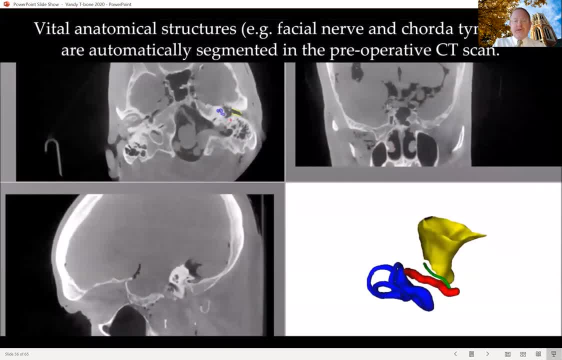 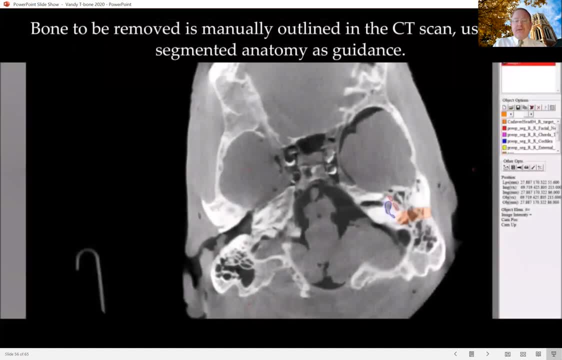 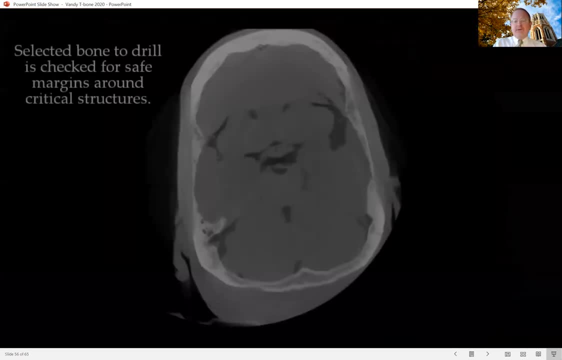 This is another project we're working on that we're doing in the cadaver lab where we physically attach a robot to a skull to do a translabyrinthine approach. First we do planning of what we want to remove. So you can see in orange all of this material to be removed by the robot. 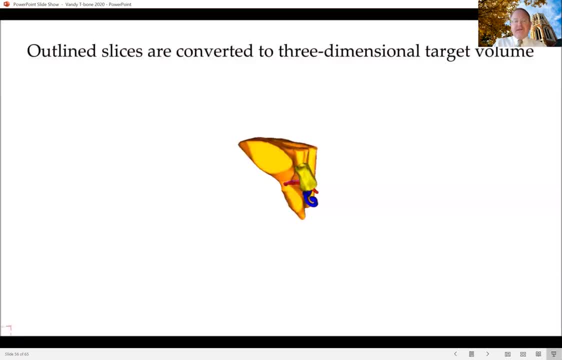 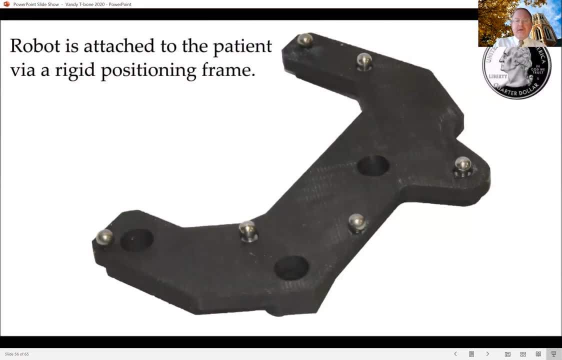 We want to make sure that we don't contact the vital anatomy and we have adequate safety margins. The surgeon has to review this, confirm that it is indeed the amount to be removed. This is a pre-positioning frame that attaches to the patient. 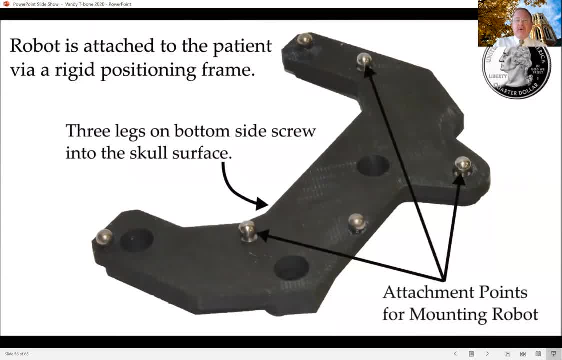 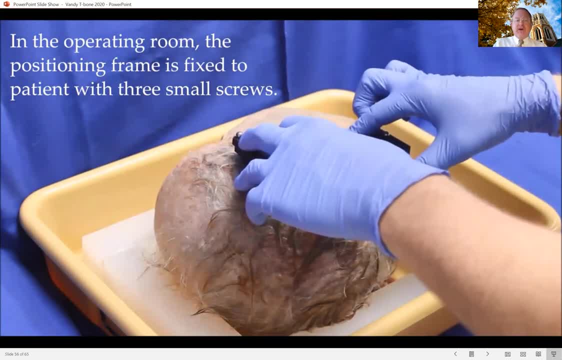 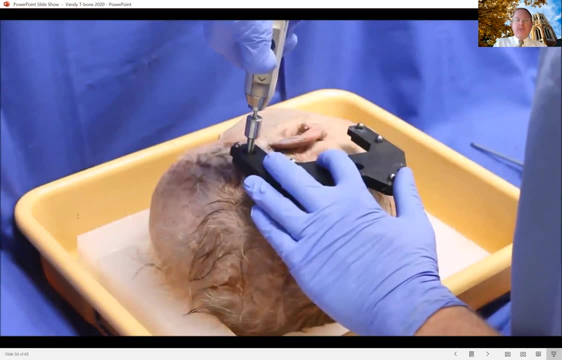 The spherical metal markers here serve both as fiducial markers for localization and also the attachment points for the robot. We place the positioning frame on the head, leaving enough room for access to the lateral skull base for both the robot and the human operator. 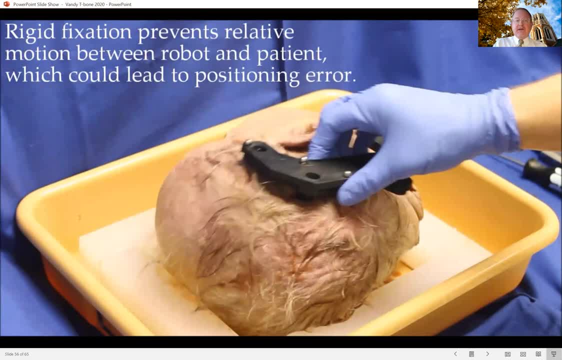 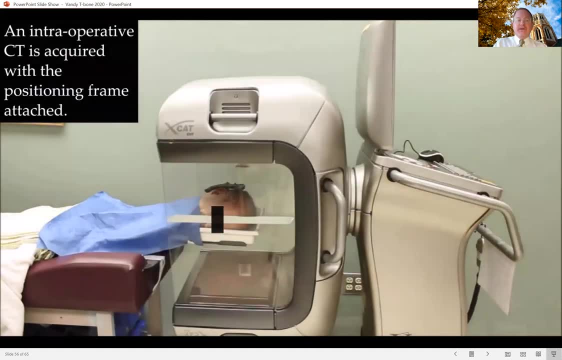 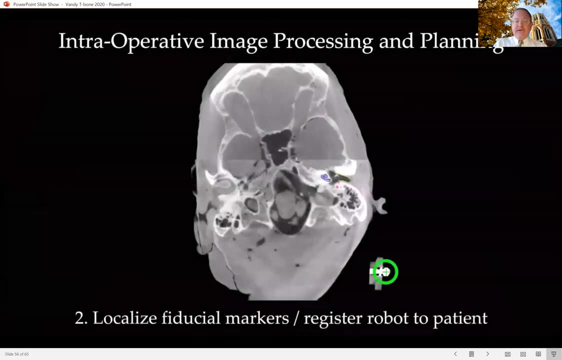 After this is attached, we take a CT scan, again using that intraoperative CT scanner, which will show us where the fiducial markers are in both CT space, and we'll pick those up in the operating room and link them together. So now we've found those markers. 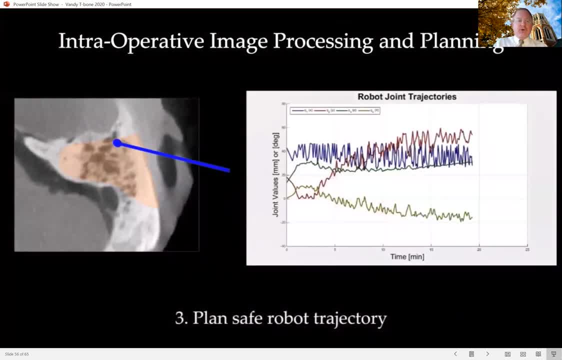 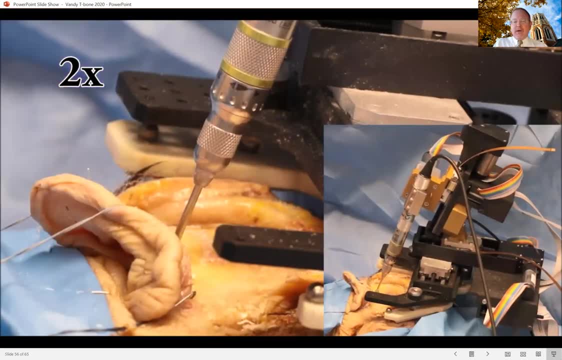 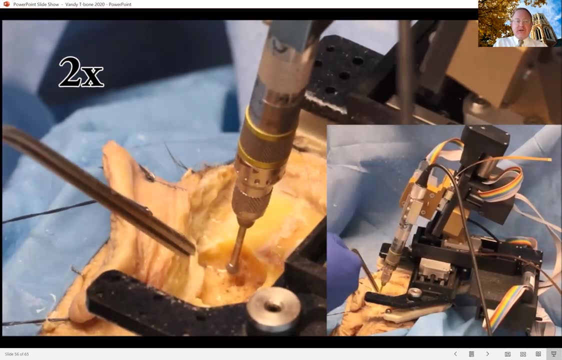 We're going to do a little bit of kinematics work with the robot to ensure that it doesn't fold over itself, And then we're going to attach the robot to the pre-positioning frame and we're going to start to drill. And it's interesting on this that the suction irrigator 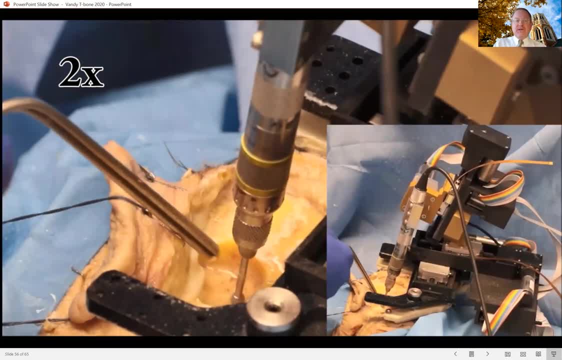 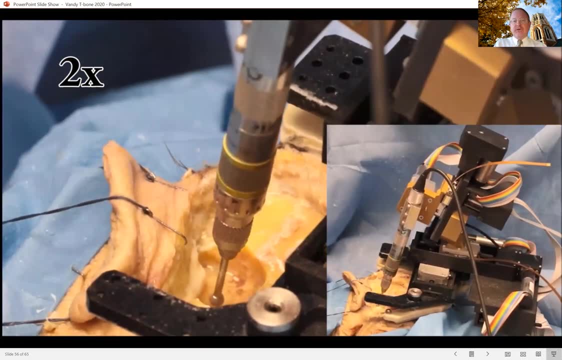 that's being held by the human being is there only so you can see what the robot's doing, because the robot knows where the tip of that drill bit is in relationship to the fiducial markers, which is then in relationship to the patient's anatomy. 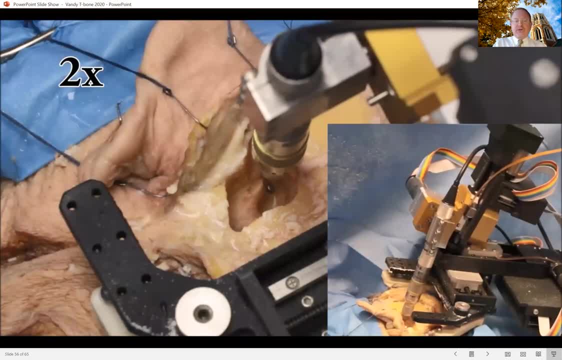 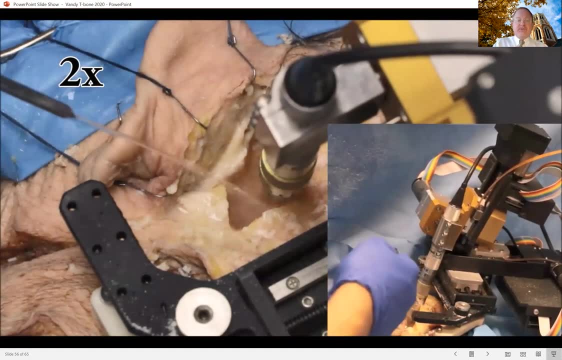 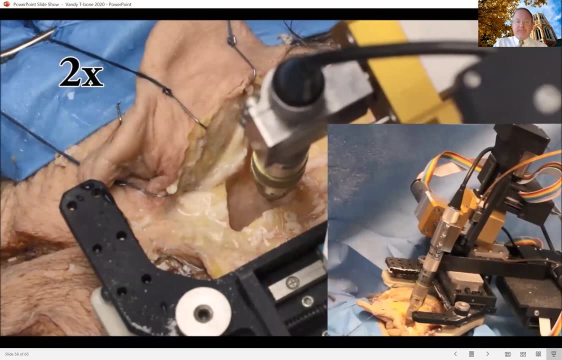 And as we go down below the cortex, we will start to drill behind the facial nerve and do the translabyrinthine approach, And the concept for this is that this would free up a surgeon to be able to do the vital work, the delicate work of the IAC: teasing off the tumor. 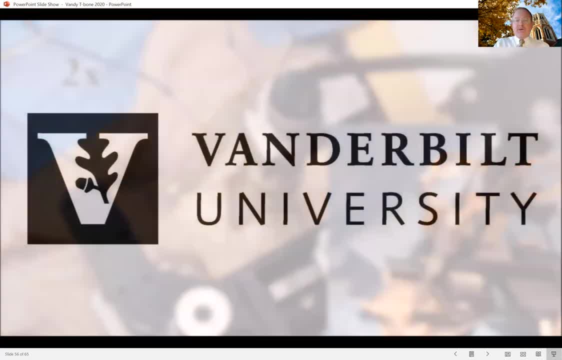 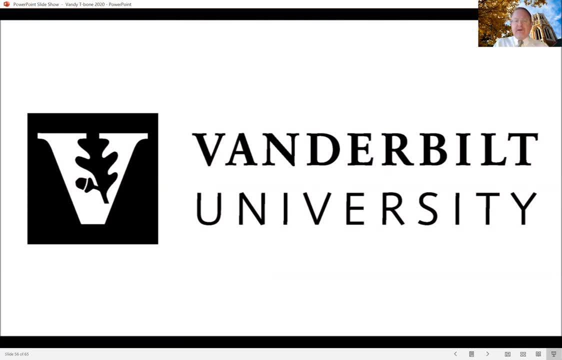 To do this right now in the cadaver lab, once the robot is attached, takes approximately one and a half hours, But with better PLATH planning we think we can get that down to about 30 to 40 minutes. So imagine if you will. 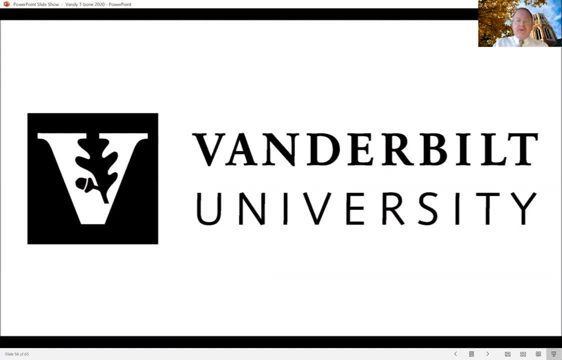 that you're in the operating room and you attach this and 30 minutes later you are doing the nice dissection in the IAC with your neurosurgical colleagues. I think it would make for a quicker day, So hopefully I've covered these three things. 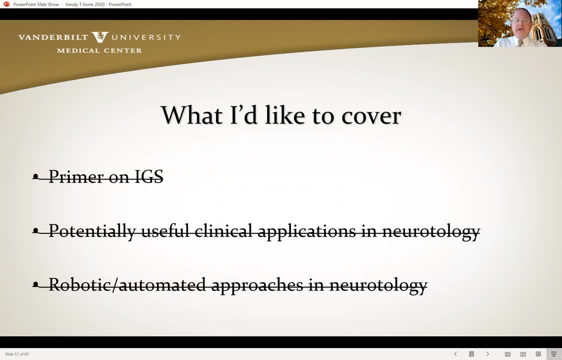 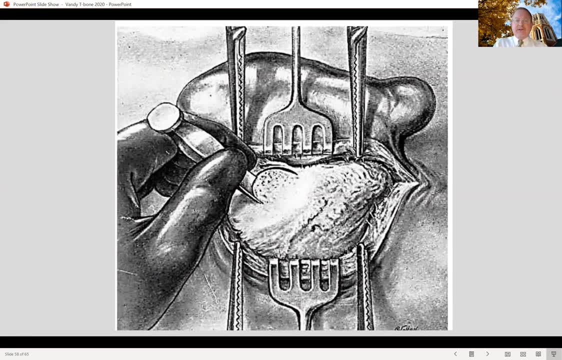 primer on IGS- useful clinical applications- and then offered some insights into what the future holds for us. If we take a look back on technology, this is where we were in the 1950s. It's really hard to believe that we were really using 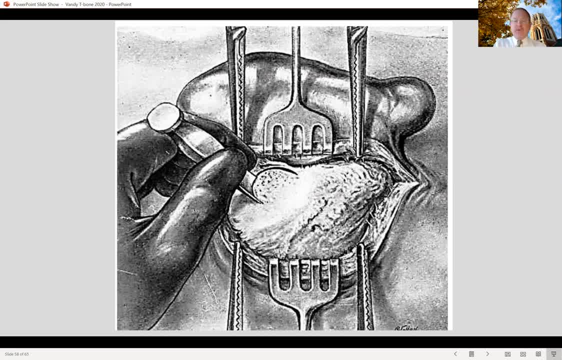 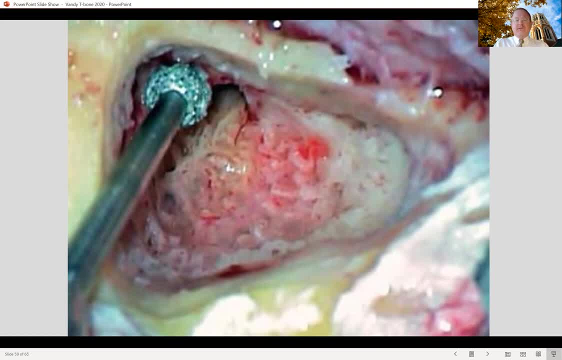 chisel and hammer to do a mastoidectomy. but we were- And it was a number of innovators- Julius, Lempert and the Hauses who really helped us evolve- to using surgical drills so that we could do the same surgery. 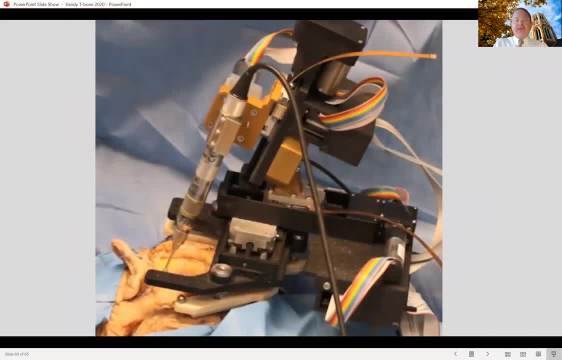 We're kind of at that junction now where we have this robot that can do the same thing, And, from an engineering standpoint, when you ask an engineer what's better- a robot or a human being- Well all you have to do is look inside a factory line. 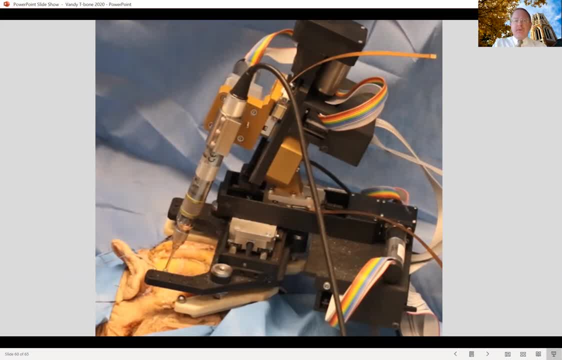 at an automobile plant and you'll see that robots are doing the job because they're more reliable and they're more accurate, And patients come to us, and I think this is a carryover from urology and the da Vinci surgical system. 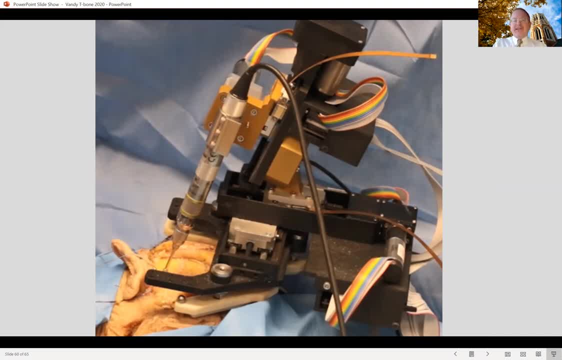 and they want a robot to do the job. They think that that technology is better And really this technology is a tool for us as surgeons and we have to be ready to capitalize on that. And central to all of that, of course. 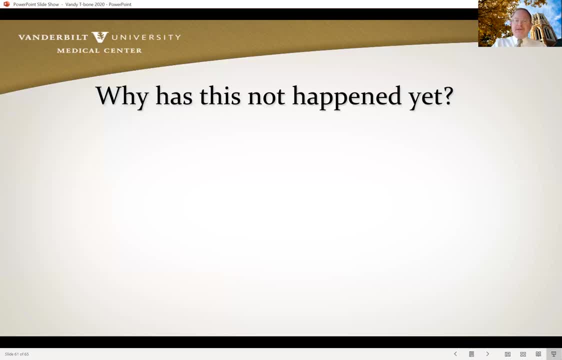 is understanding image guidance. So why is this not happening yet? Again, I don't know, but I really think it's coming and I think we need to be prepared for answering questions to our patients, for being in the operating room and getting the best accuracy. 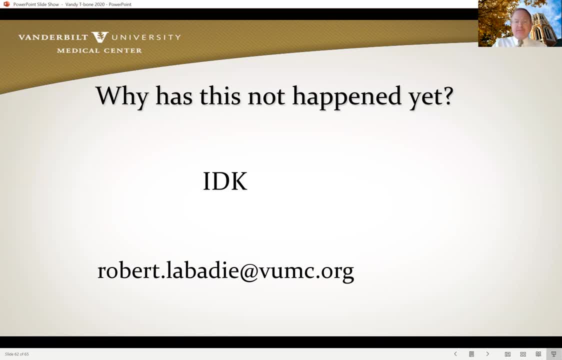 that these systems can achieve. Thank you so much. Here's my email if there's any questions, and I'll be available in the panels. I'll be happy to answer questions as they arise.